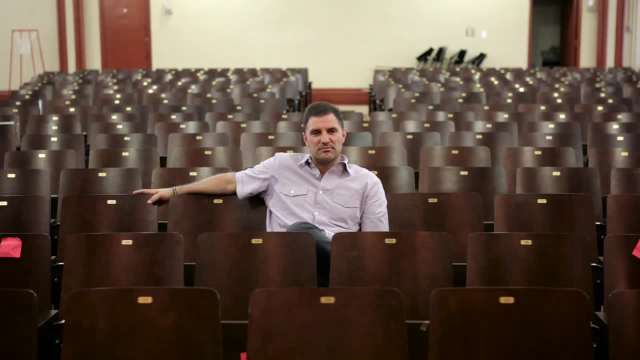 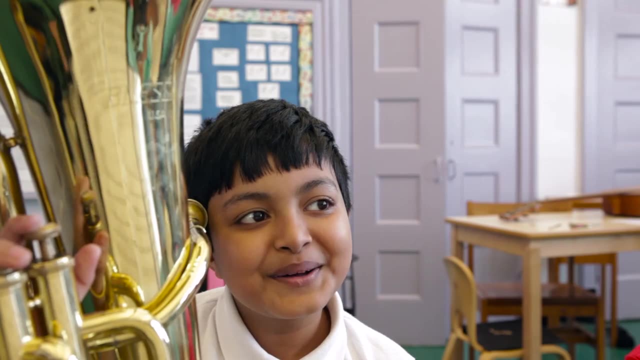 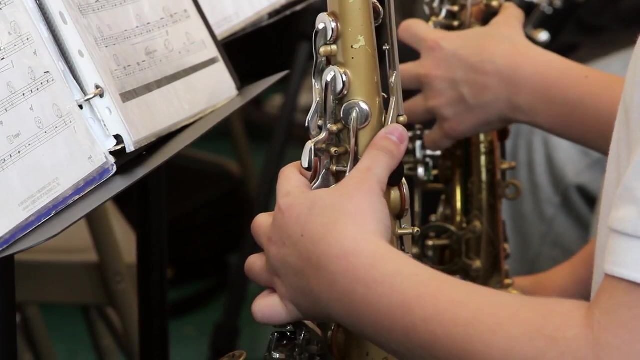 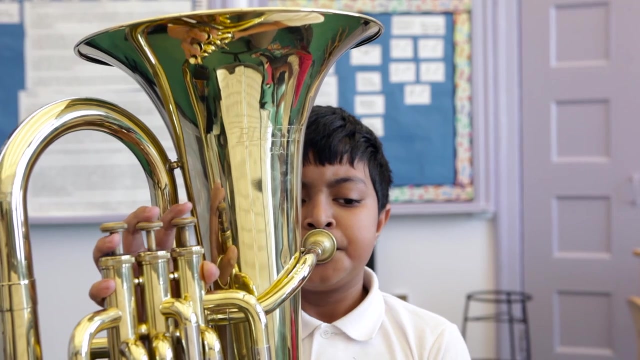 We're going to rock it out. We'll be okay. The students come on their lunch, We start rehearsing and we practice for like half an hour Now. obviously we're working on our repertoire. We keep pushing the envelope to try to do more and more and more. 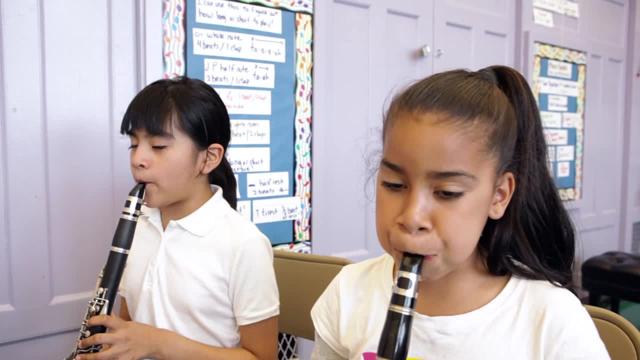 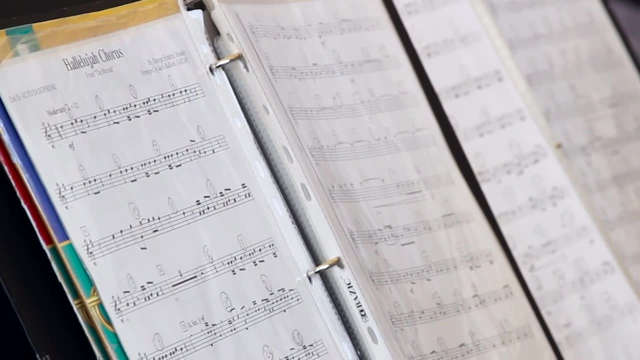 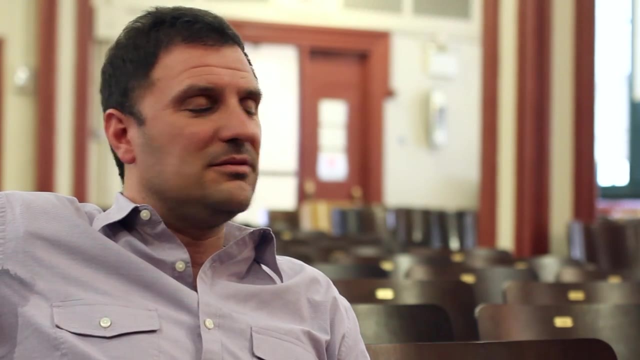 There's an art making going on that's just unbelievable. We have nine and ten year olds performing Händel, A piece written in 1740 that I didn't learn until I was 31.. They're learning it at nine. It's awesome. 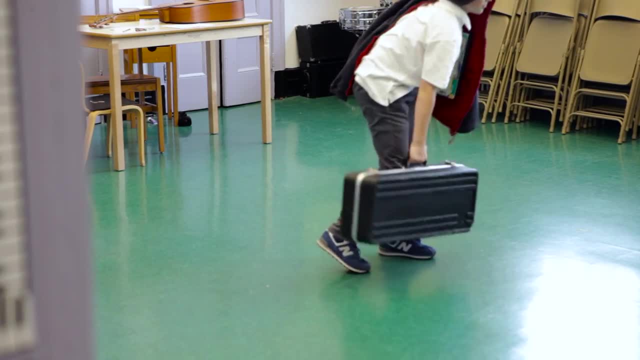 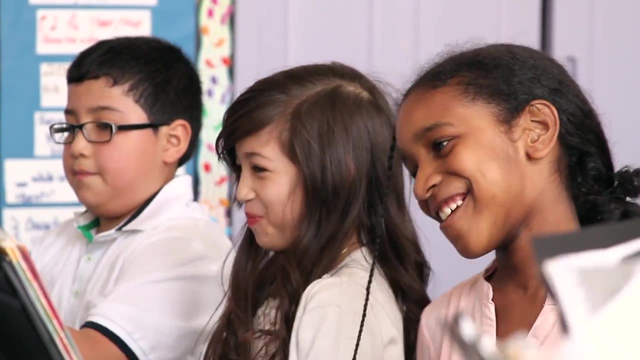 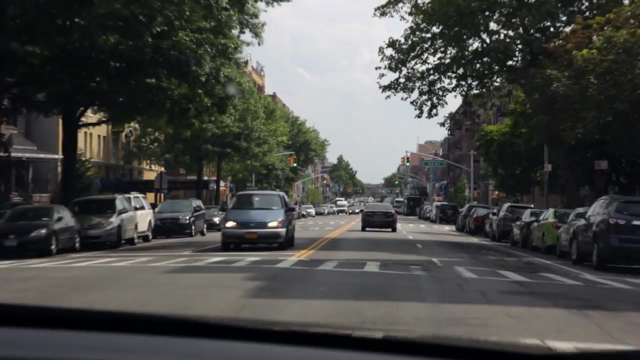 Most elementary school programs don't meet every day. They meet once a week. My students: they're trained as musicians. They give up being outside, They give up being playing. It's huge, Tremendous sacrifice. Borough Park: I feel very safe here. 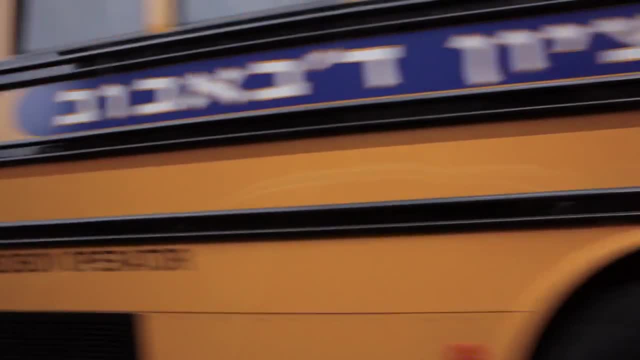 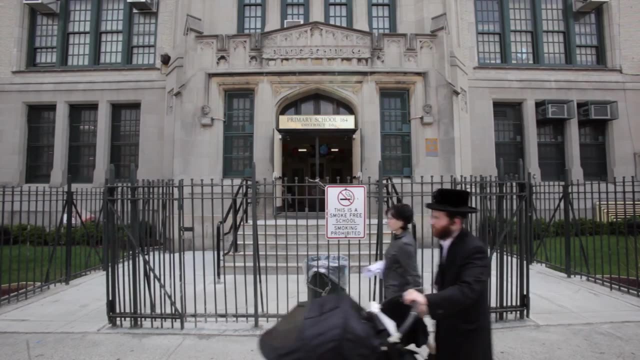 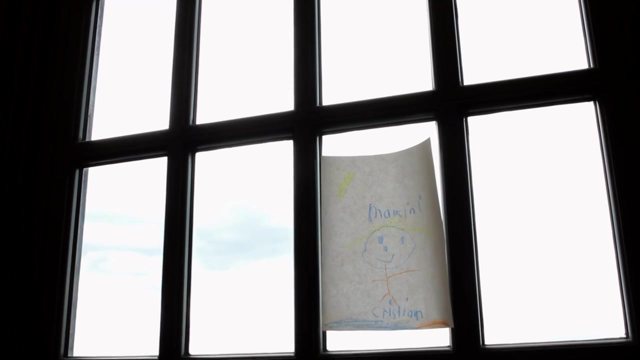 I don't know. It just seems like it's separate from the world. here We're in Brooklyn, but it seems like we're someplace else sometimes. My students are all immigrants, Children of immigrants: The Bengalis, the Spanish, the Mexicans, the Uzbekistan, some Polish kids from all parts of the world. 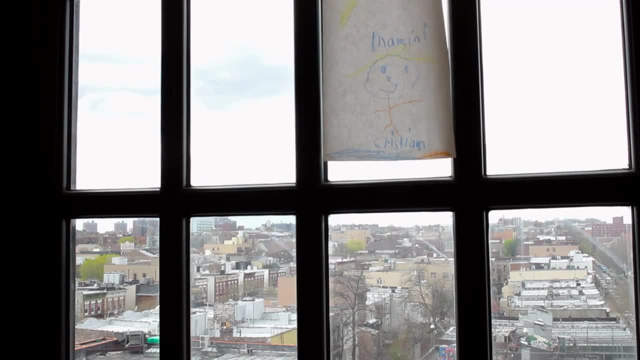 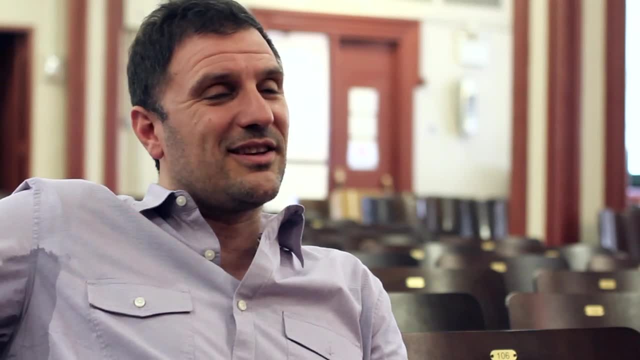 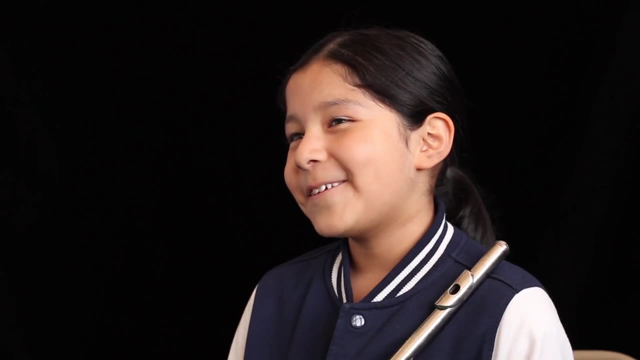 Doing things that are extraordinary. I became a music teacher because I love music. I really get a chance to infect in a good way children's life with music. If I had to describe Mr Mancini, He's very unusual. 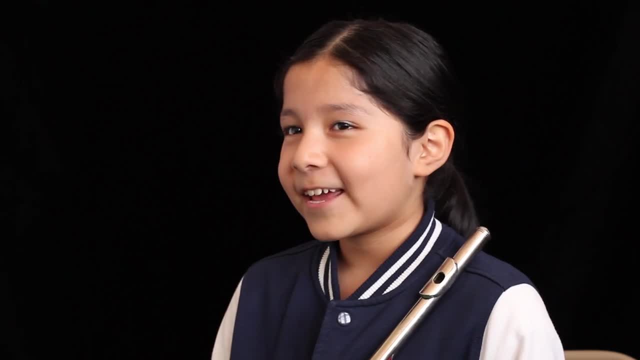 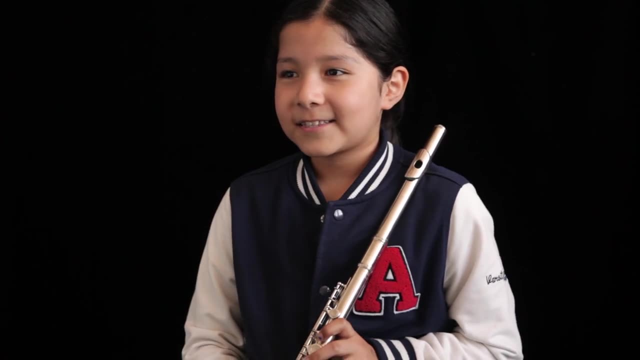 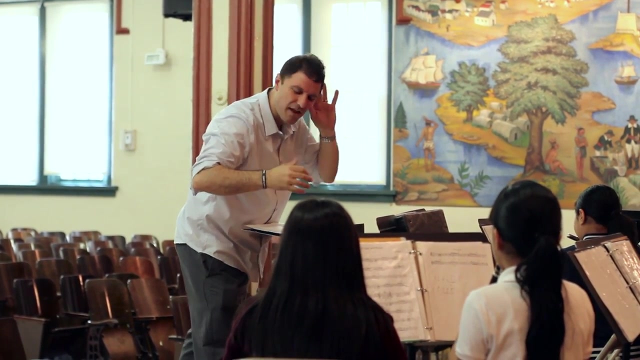 Hardworking. funny. He's not like a normal music teacher. I played it right? No, It's not. He teaches us different things about music And it sort of relates to our schoolwork. He pushes you really hard so that when you grow up and keep playing music, you still have those tips that he gives you. 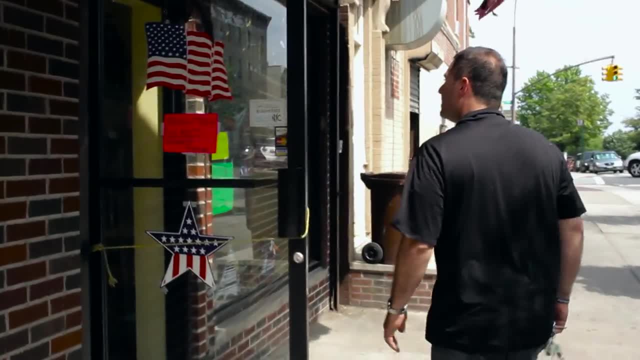 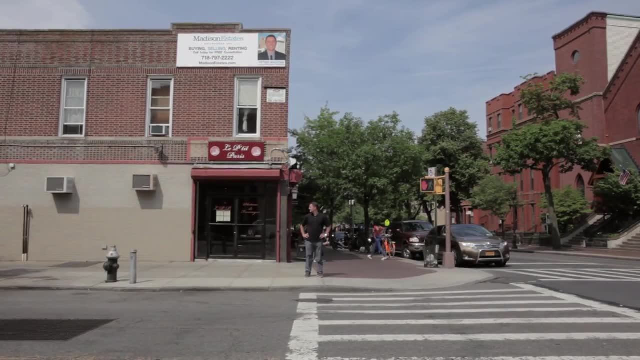 My mom and dad are from Mola di Bari, Italy. They came over on the boat You left. your father Grew up basically in an Italo-Americano area. I came to work here. The bakery used to be the entire property.